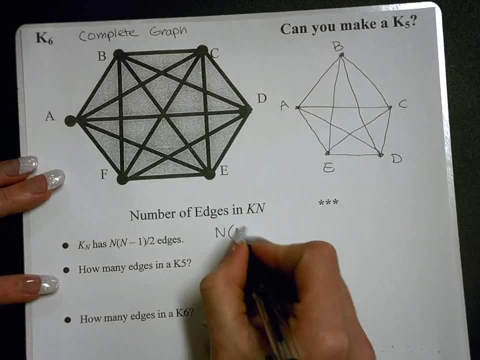 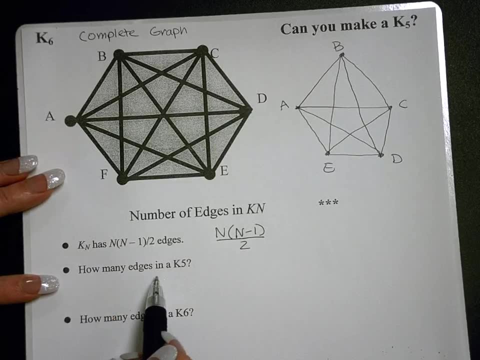 The formula is N multiplied by the quantity N minus 1,, all over 2, and for K, N, N denoting how many vertices are in the complete graph. So what we're going to do is we're going to find out how many edges are in this K-5.. 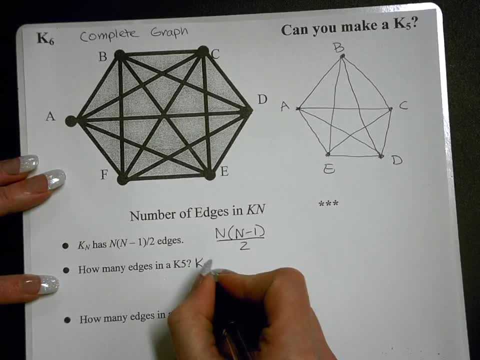 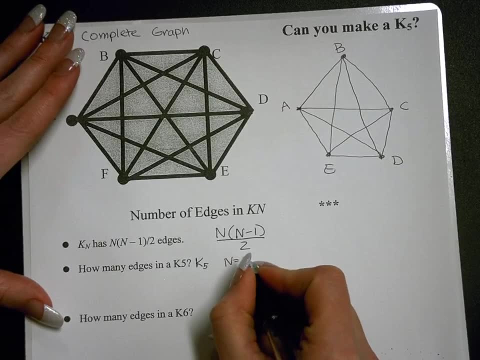 So when the K-5, This symbol is actually written a little bit, that 5 needs to be subscript. So then this 5, that's what n equals. so I'm going to say n equals 5.. Then what we're going to do is we're just going to plug 5 into this formula to figure: 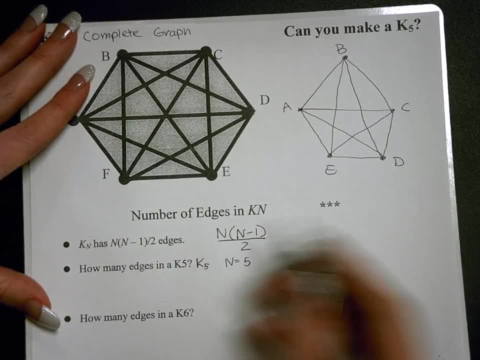 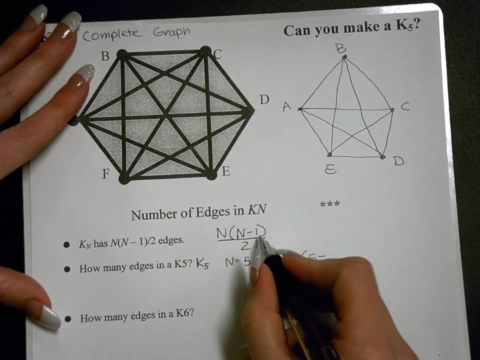 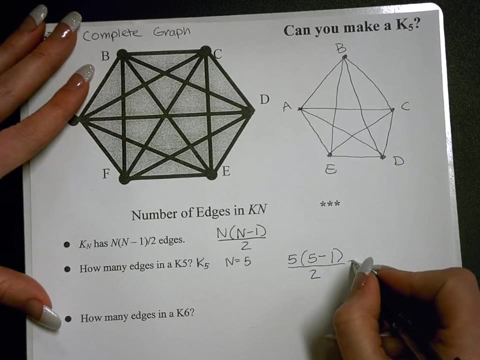 out how many edges are in this K5.. So right here is an n. so I'm going to write 5 and then parenthesis, and then 5 minus 1 parenthesis, all over all divided by 2.. Now I'm just going to use order of operations. 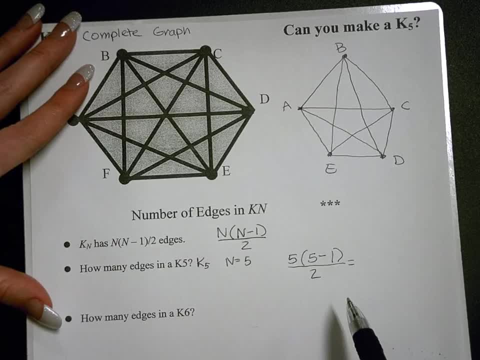 Order of operations. remember parenthesis: exponents, multiplication, division and then addition and subtraction. See, we have parenthesis here. so that's the operation that we're going to do first. We're going to do 5 minus 1.. 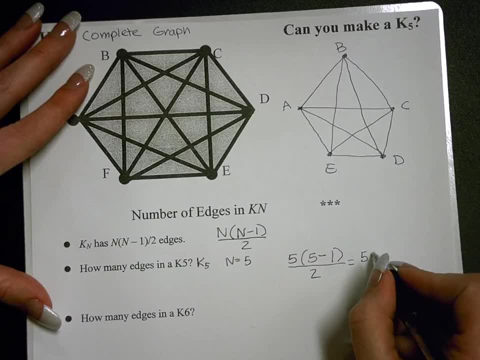 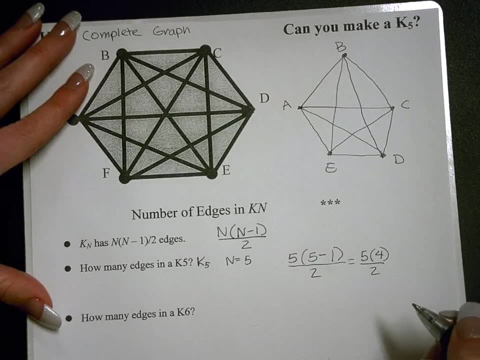 We're going to rewrite everything else. So I'm going to rewrite this: 5,, 5 times. well, 5 minus 1, what is that? That is 4 divided by 2.. Okay, And then I'm going to do just the simplification, the multiplication and the division. 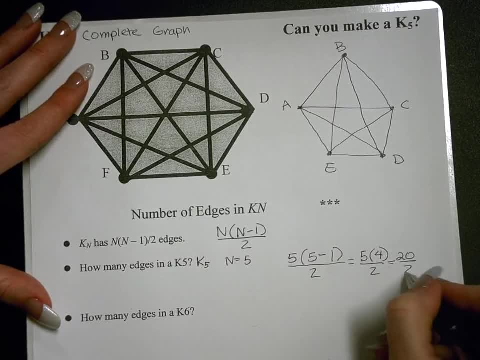 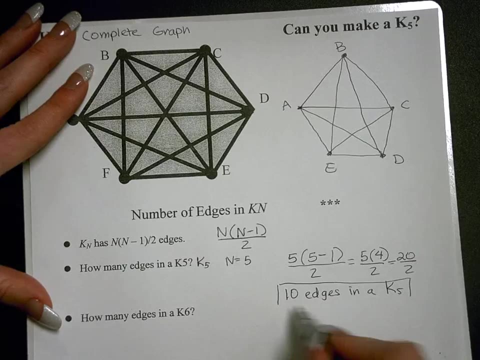 So 5 times 4 is 20 divided by 2. And 20 divided by 2 is 10.. So that means there's 10 edges in a K5, a complete graph that has 5 vertices. Now let's practice this process one more time, but with a K6.. 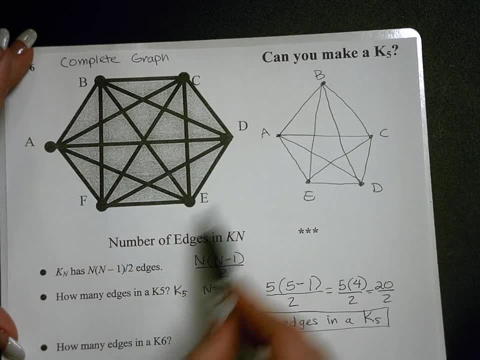 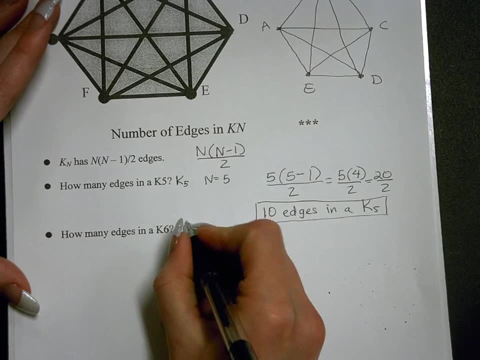 This complete graph up here. This isn't exactly. this is a K6. So let's see how many edges are in this K6.. I'm going to rewrite this symbol. It's K6 with a subscript 6.. That means that n is equal to 6.. 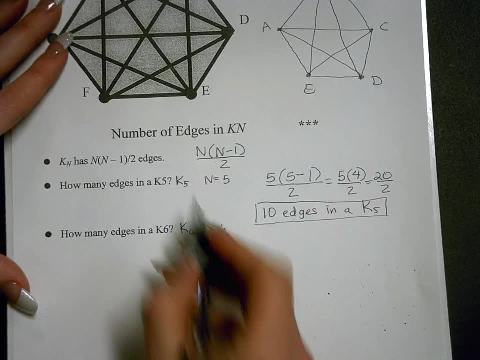 So I'm going to use this formula. I'm just going to plug in 6 where there's n, So there's an n, so I'm going to put 6, parenthesis, 6 minus 1, parenthesis, all over.